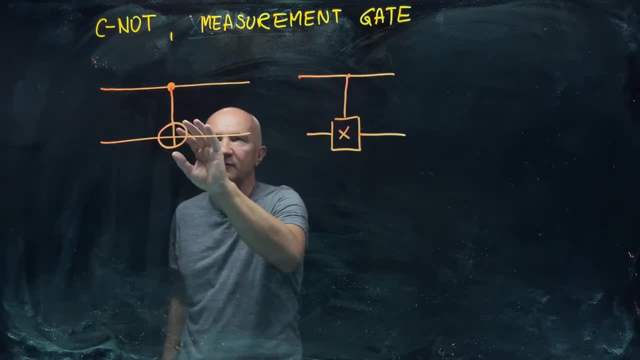 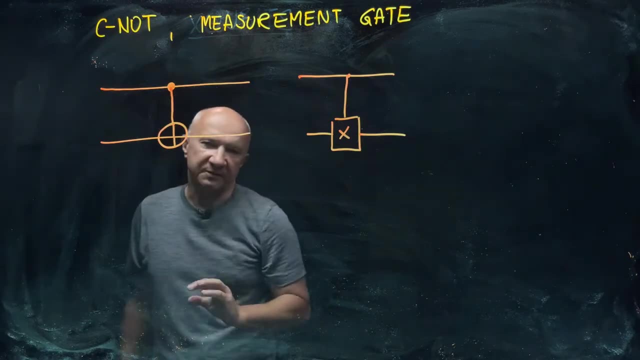 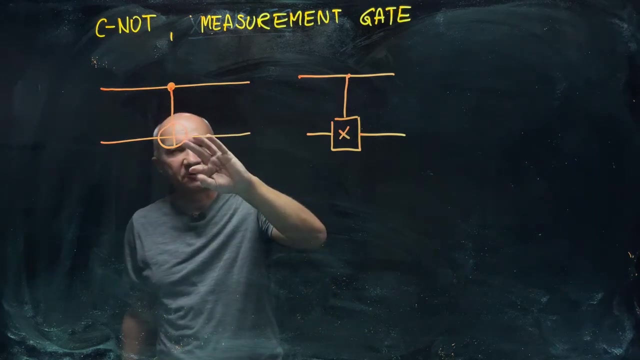 unitary operations applied to the, the second, the target qubit. In this case, if the, the first qubit is in the state zero, then nothing happens to the second qubit, And if the first qubit is in one, then operation logical, not or bit flip is applied to the second qubit. So that's why you 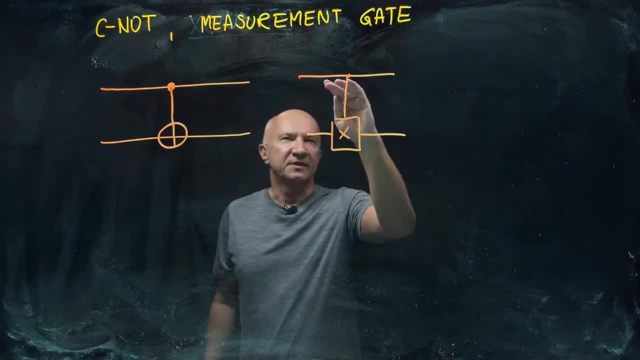 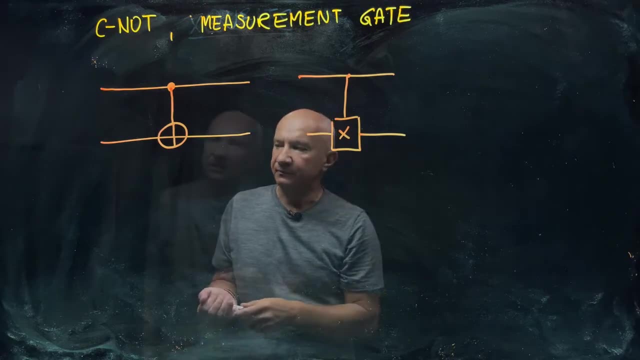 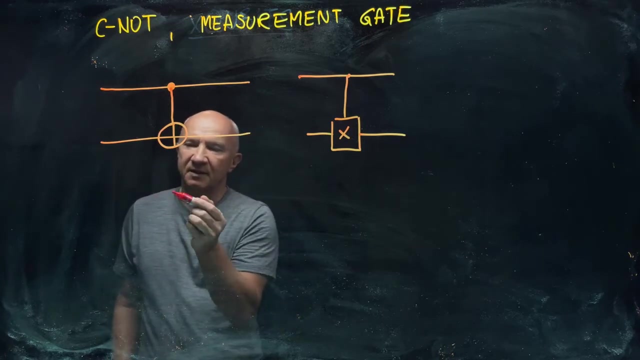 have alternative diagram here which essentially says the same thing, and an X here stands for the X gate, single qubit X gate or a bit flip. So the the action of this gate, if we want to be a little bit more specific, is can be just completely specified. 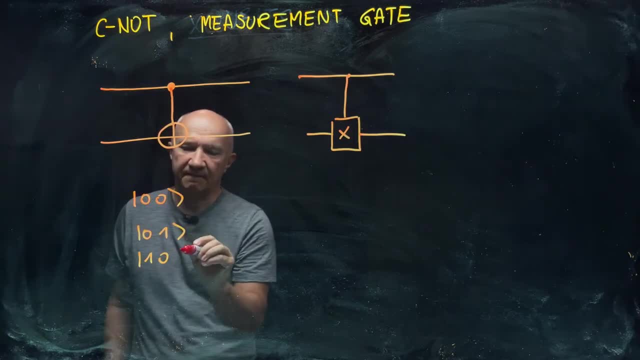 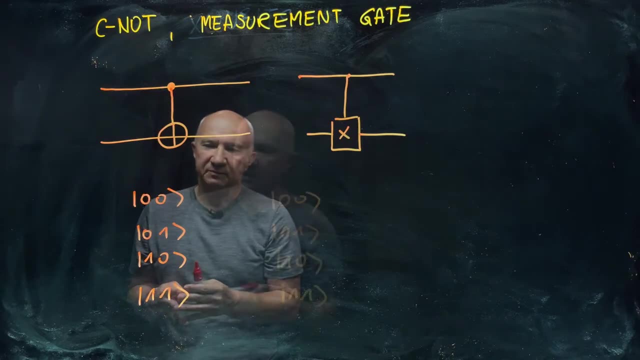 if I tell you how it acts on the, on the four basis state. So I have four basis states of my two qubits. So the first qubit is the control qubit, the second one is the target qubit. So if the first qubit is 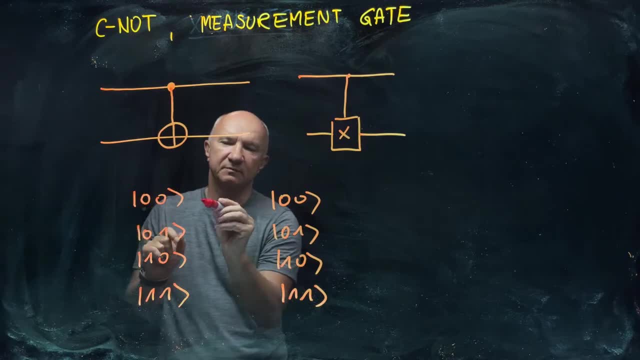 in state zero, nothing happens to the second qubit. Now again, if the first qubit is in state zero and the second one is in state one, well, again, it doesn't matter, because the first one is in state zero, we apply the identity. nothing happens to the second qubit. Now, if the first qubit is in 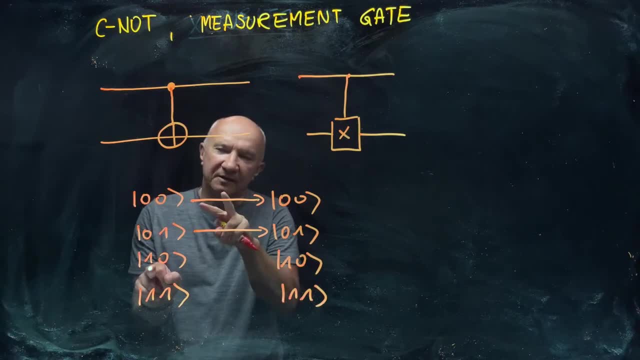 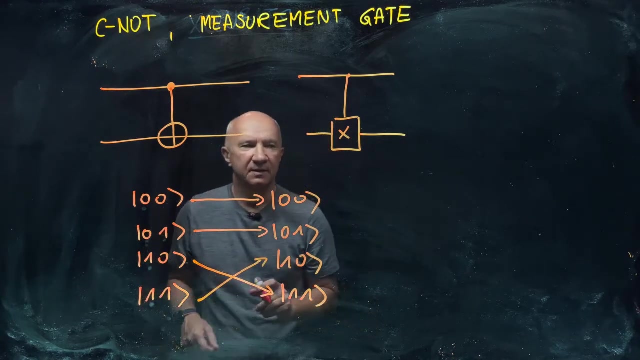 state one, then we apply the bit flip, So that means zero on the target. qubit becomes one. So this one goes into this one and, as you can see, this state is mapped into this state. So there are other ways of writing this. you can you. 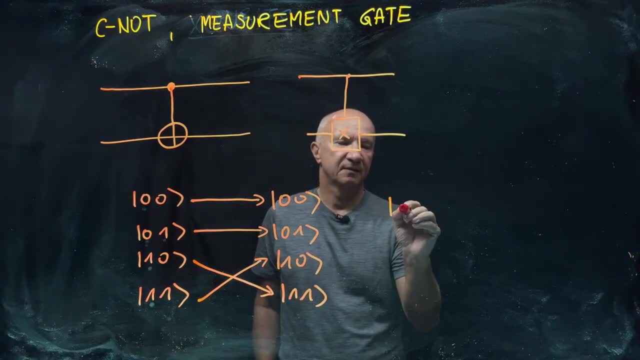 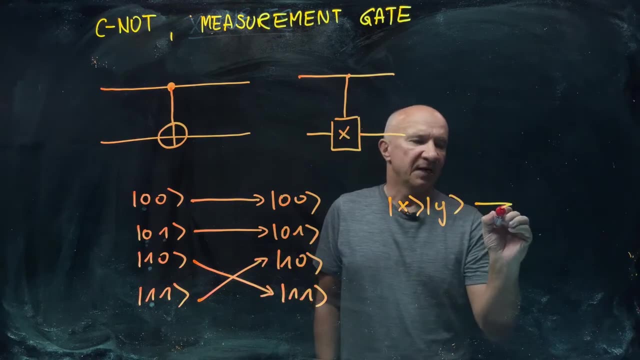 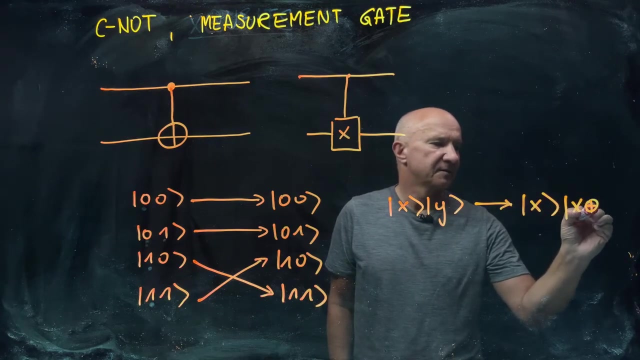 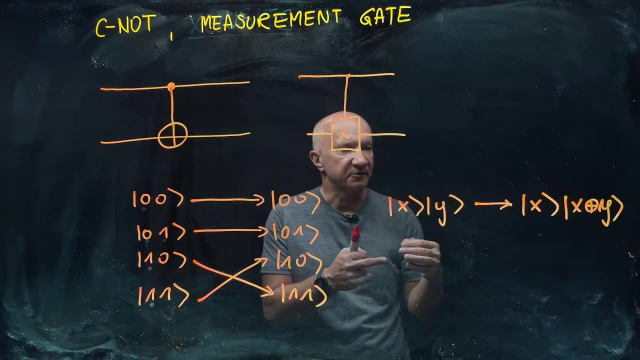 can write it as follows: State x- y, where x and y are either 0 or 1, is mapped into a state x. You see, x always survives, and here you have x and that's binary addition, x plus y, So that's exclusive or binary addition. So that means that you know 1. 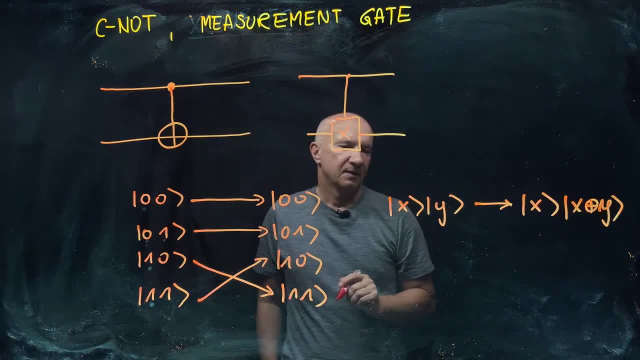 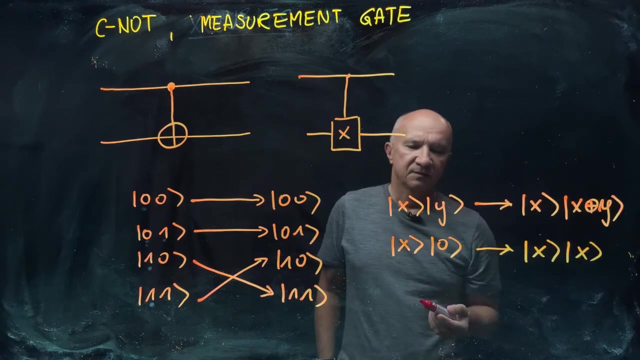 plus 1 is 0 in this case, And in particular if y is equal to 0. that's that's kind of interesting case that we will look at later on, and this will be mapped to x- x, So somehow the the state of the qubit. 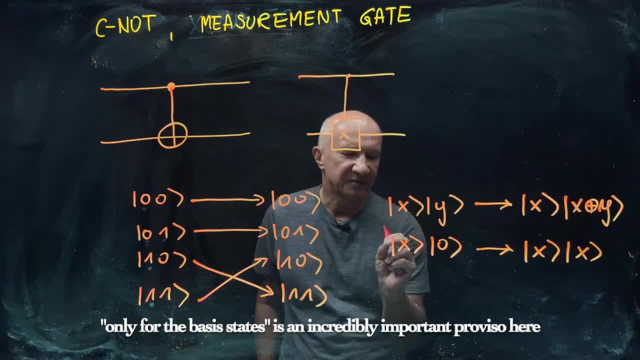 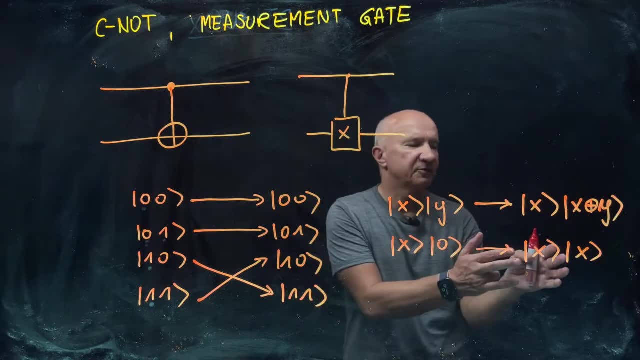 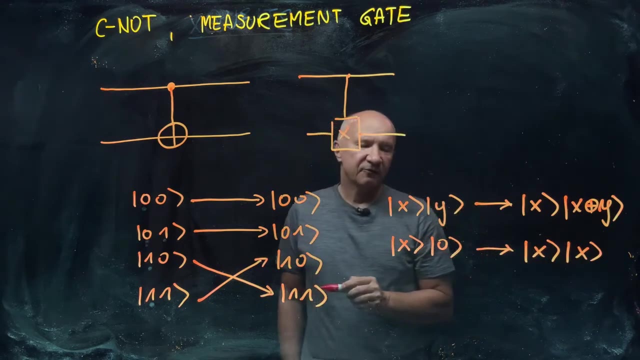 but again only for the basis state, only when x is equal 0 or 1, the state of the qubit of the first qubit is just copied. so then you have a copy of the of the first qubit, So we will start on the second qubit as well. Yet another way of writing this is: 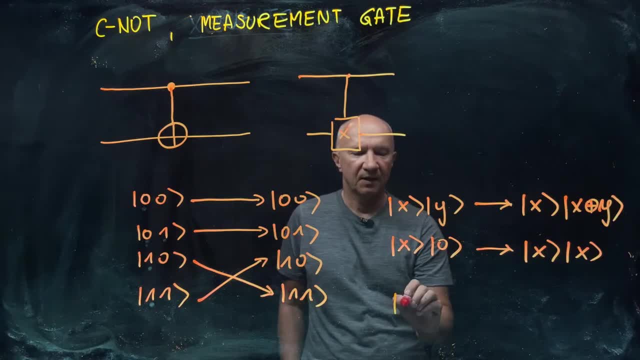 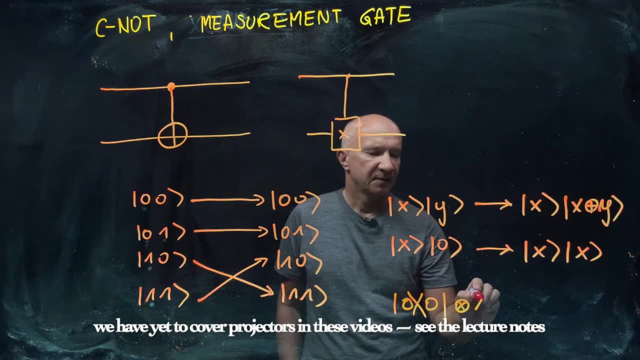 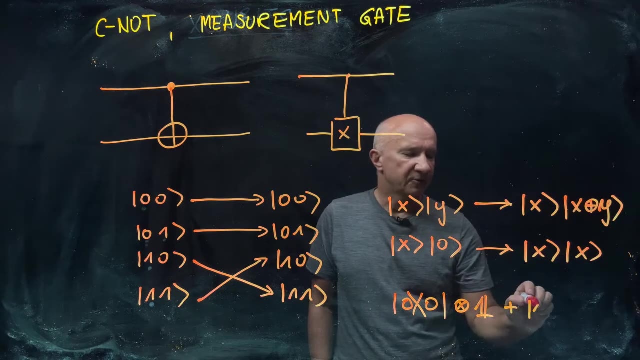 this. this gate is as follows: We say: well, okay, if the first qubit is in state 0, it's a projector on 0, then do nothing to the to the second qubit or your target qubit. however, if your first qubit is in state 1, 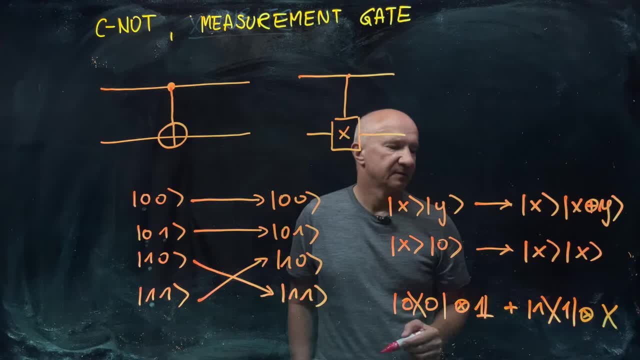 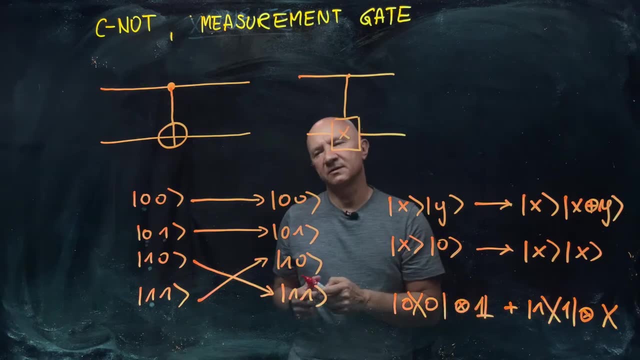 apply operation X, the bit flip, to the second qubit. so that's, that's another way of writing this, this, this operation, and of course, you know, if you really want, you can use this basis and you can write it as a matrix as well. so you can. 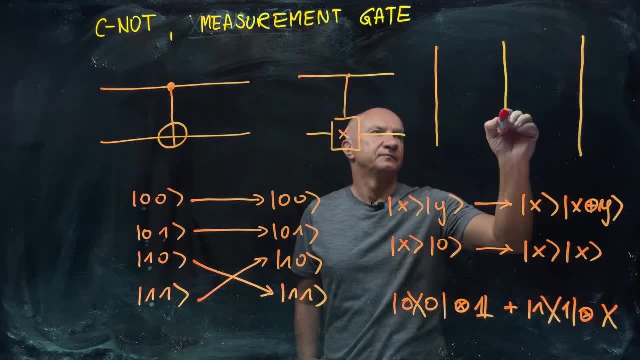 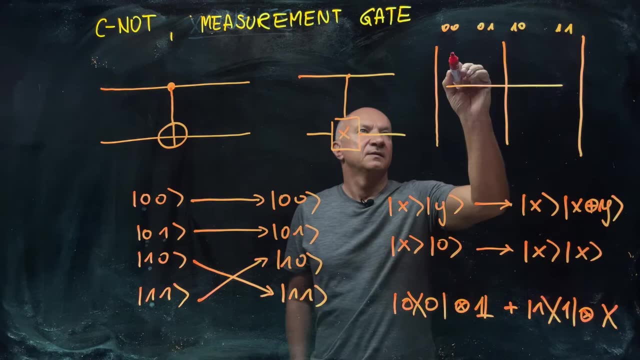 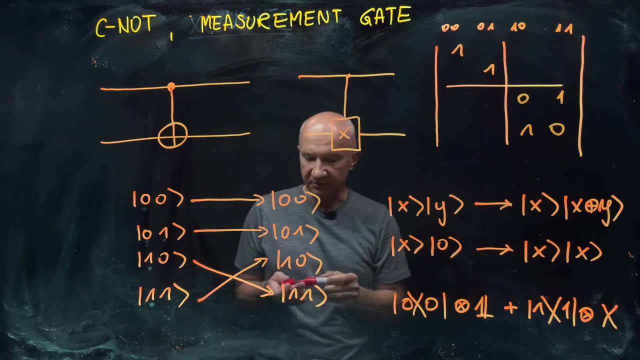 in this case you will have, if those are state 0, 0, 0, 1, 1 0 and 1: 1. so this matrix will look like like this and, of course, zeros on the L diagonals. so you have. you have now a good characterization of the most popular two. 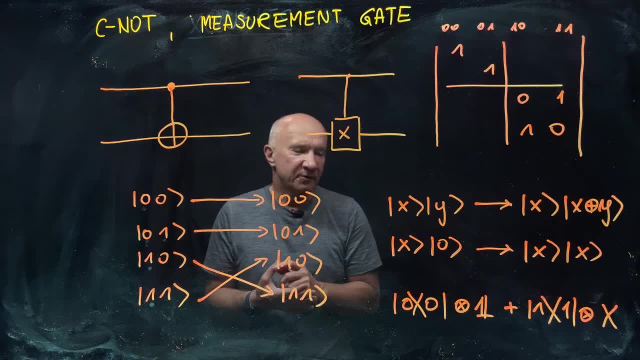 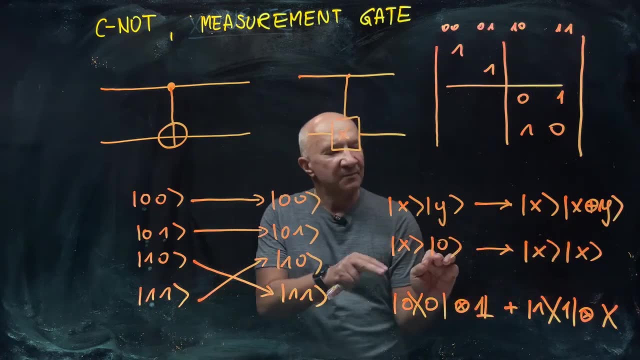 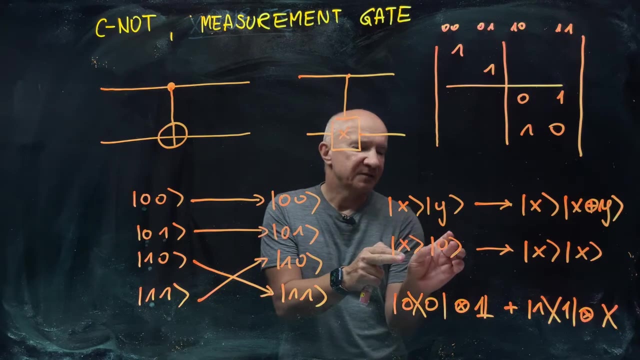 qubit gate, control, node gate, all the measurement gate, the measurement gate of the measurement gate is the measurement gate, measurement gate. the name refers to this particular scenario where somehow, when you start in the in the X zero state, so you prepare the second qubit in state. 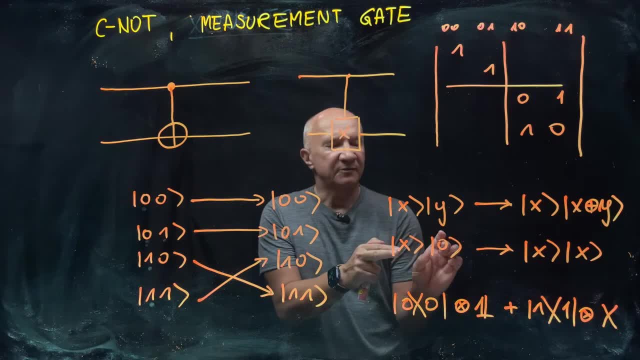 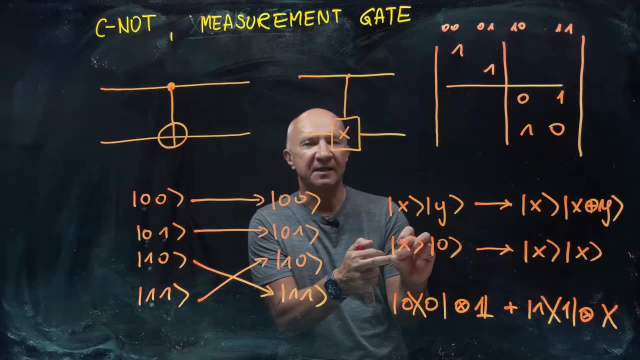 zero, then you can think about it as a, as a, as a measuring qubit. the qubit is prepared in state zero and wants to learn the state, the basis state of the first qubit. that could be either zero one, so the the second qubit is thinking: